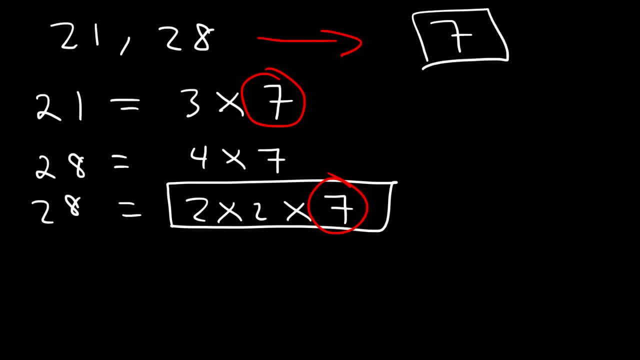 The answer is 7.. Now let's work on another example: 22 and 55.. Go ahead and pause the video. Find the GCF. the greatest common factor between these two numbers, 22, is 2 times 11.. 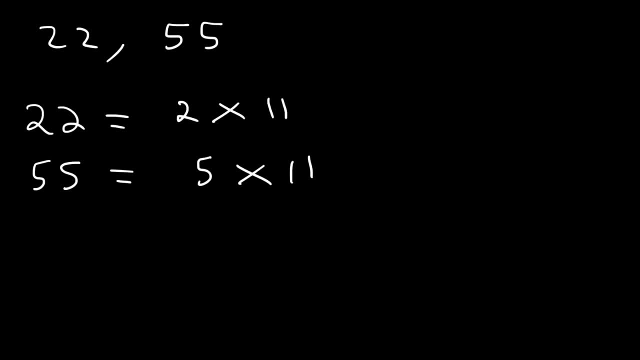 55 is 5 times 11. The GCF is 11. Find the GCF between 12 and 16. So take a minute, pause the video and work on that example. So 12 is 4 times 3.. 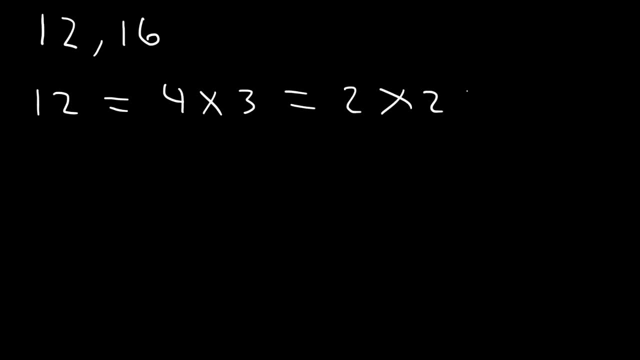 And 4 is a composite number which we can break down into 2 times 3.. So that's the prime factorization of 12. And for 16, which is 4 times 4.. 4 can be broken up into 2 times 2.. 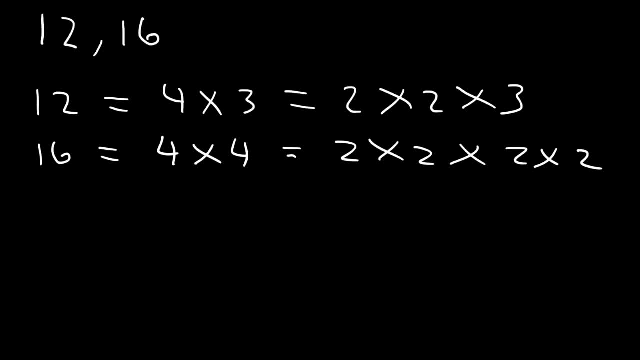 And the other 4 is 2 times 2 as well. So it takes 4 twos to get to 16.. Now that we've written the prime factorization of 12 and 16, we can identify the greatest common factor. 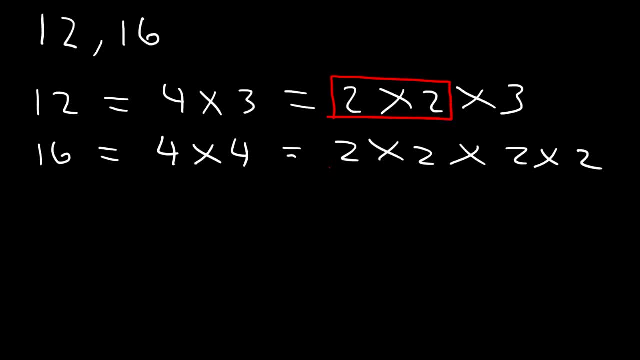 So the first number have two twos, The last one also have two twos. So the greatest common factor, The greatest common factor is 2 times 2,, which is 4.. Those numbers are common to 12 and 16.. 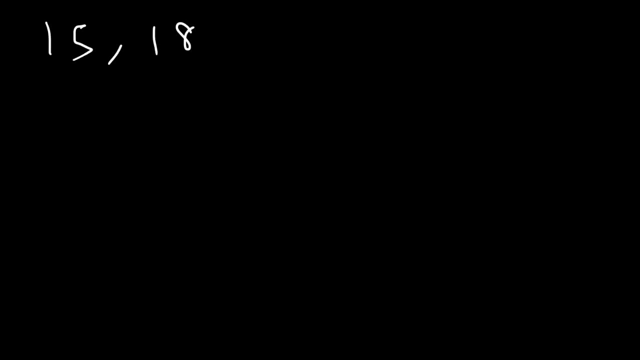 Do the same thing for 15 and 18.. Write the prime factorization and then identify the GCF. So 15 is simply 3 times 5.. We can't break it down any further than that. 18 is 6 times 3.. 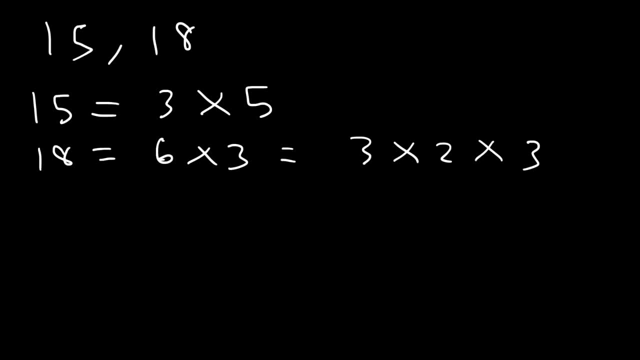 And 6 is 3 times 2. And then we still have the other 3.. So 3 is the only common factor in 18 and 15.. It's the greatest common factor, And so that's the GCF. 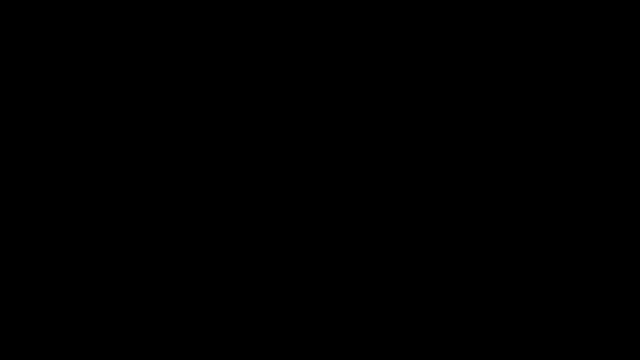 The answer is 3.. Now what about 24 and 40?? Find the GCF between the two numbers. So 24 is 4 times 6. And 4 is 2 times 2.. 6 is 3 times 2.. 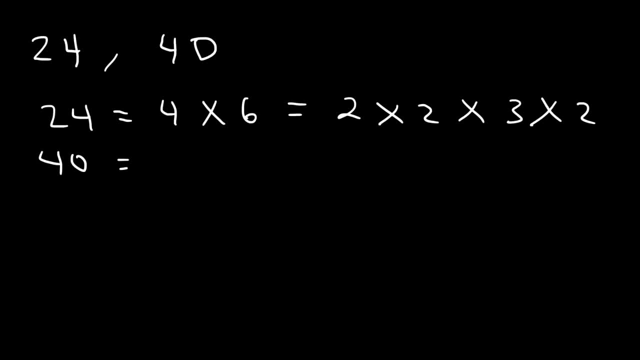 So that's the prime factorization of 24.. 40 is 8 times 5. And 8 is basically 2 times 2 times 2.. So 24 has 3 twos And 40 has 3 twos as well. 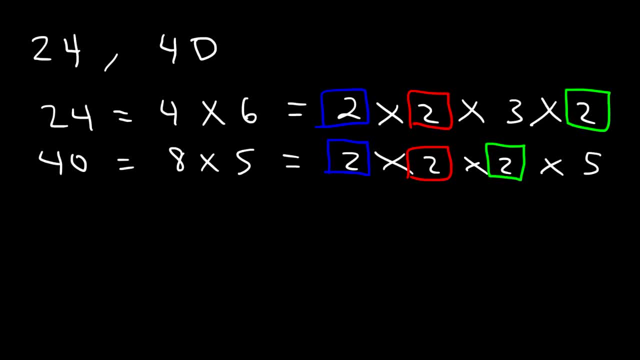 So you want to identify the prime numbers that are the same in both lists. So 24 and 40 both contain 3, twos, 2 times 2 times 2, that's 8.. So 8 is the GCF in this problem. 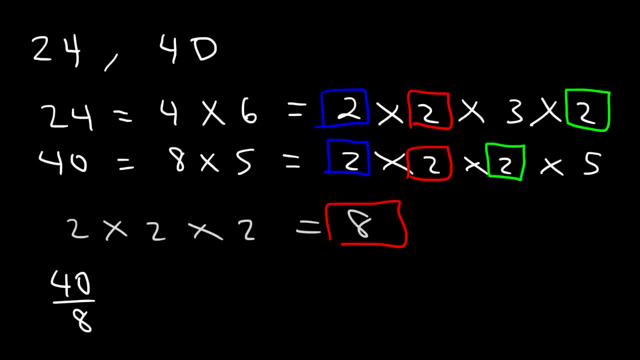 And you can check it: 40, if you divide 40 by 8, you get 5.. 24 divided by 8, you get 3.. So the GCF is going to be divisible. 24 and 40 has to be divisible both by the GCF 8.. 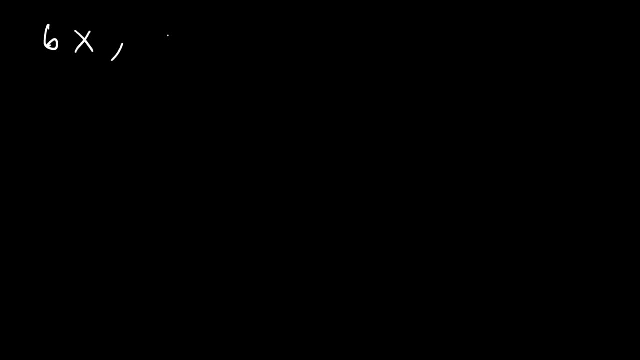 Sometimes you may need to find the GCF between two monomials, So sometimes variables will be involved. What is the greatest common factor between 6x and 9x squared? Well, the process is the same. We need to write the prime factorization of 6x. 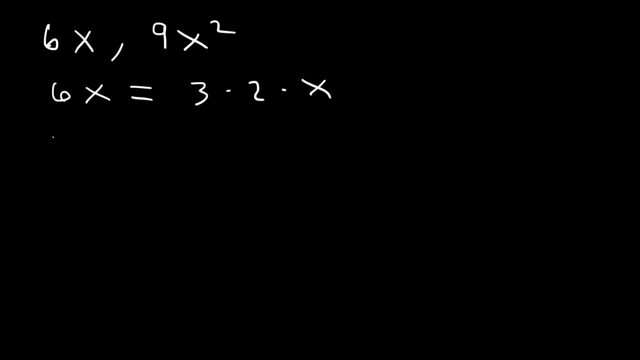 6 is 3 times 2.. And then we have an x- 9x squared. we can break down 9 into 3 times 3. And x squared is x times x. So both lists contains at least one 3 and an x. 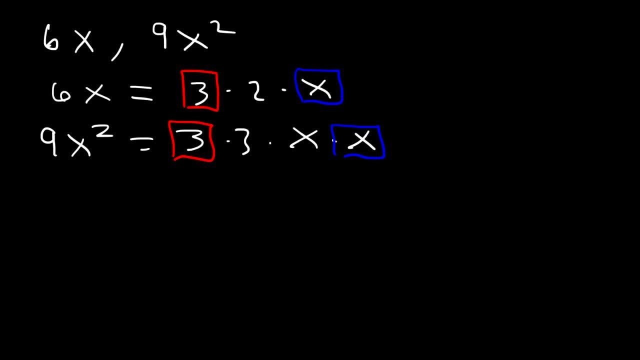 So therefore, the GCF between 6x and 9x squared is 3 times x, which is just 3x. Now what about this one, 12xy and 15x squared, y cubed? Find the GCF between these two monomials. 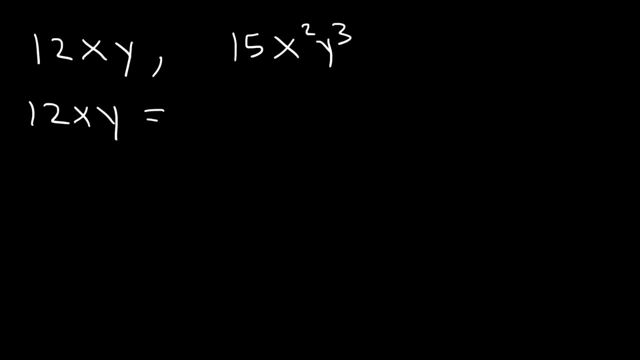 So let's start with 12xy. 12 is 3 times 4. And 4, we can write it as 2 times 2. And then we have 1x and 1y, 15x squared y cubed. 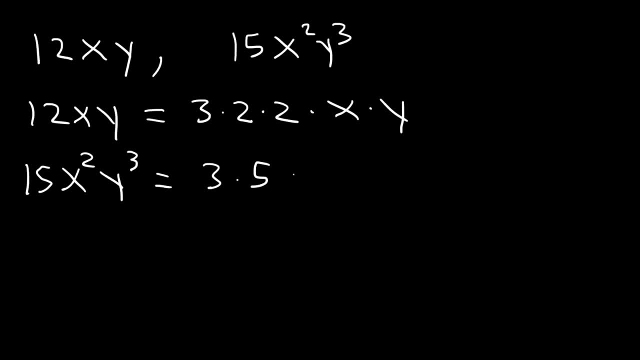 15 is 3 times 5.. And x squared is x times x. y cubed is y times y times y. So let's identify what's common in both lists. We have a 3. There's at least one x. 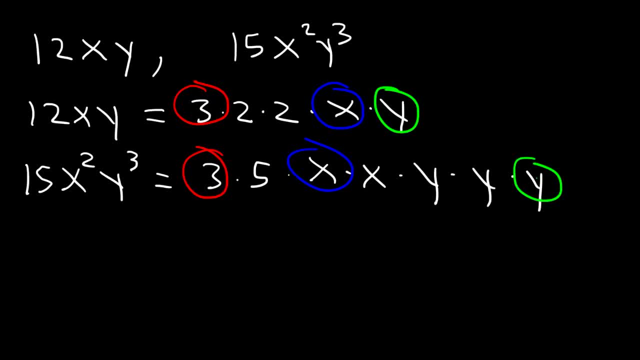 And a single y, And that's all that we can find. that's common To the two lists that we have. So the GCF, the greatest common factor, is 3xy. Try this one: 24x squared y, cubed. 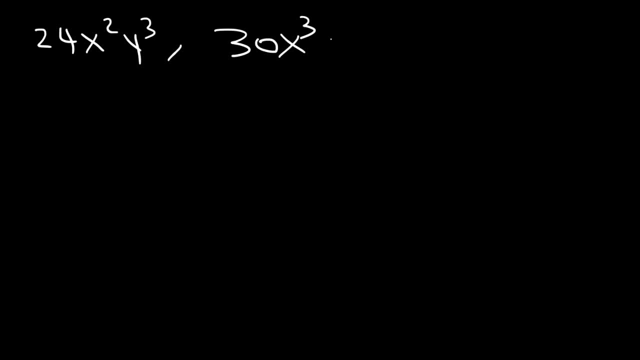 And 30x cubed y to the fourth, 24 is 4 times 6. And 4 is 2 times 2.. 6 is 2 times 3.. And then we have x squared, which is x times x. 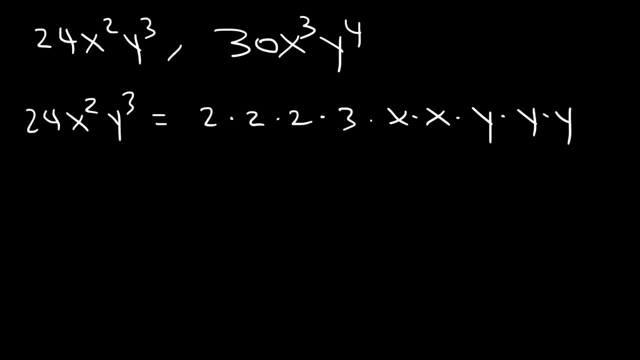 And y cubed, which is y times y times y. 30 is 5 times 6.. And 6 is 2 times 3.. And let's not forget the 5.. So 30 is 2 times 3 times 5.. 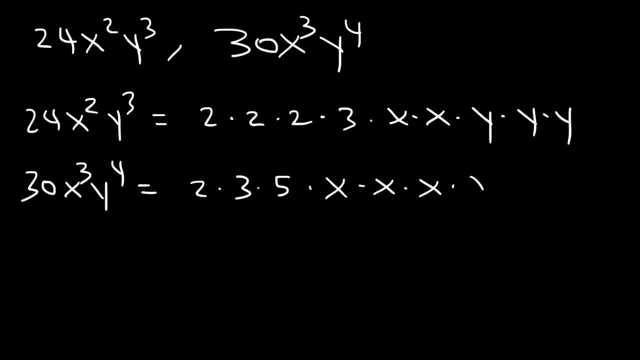 x cubed is x times x times x. y to the fourth is y times y times y four times. So 2 is common to both lists And we have a 3 as well, And then there is 2x variables that can be found in both. 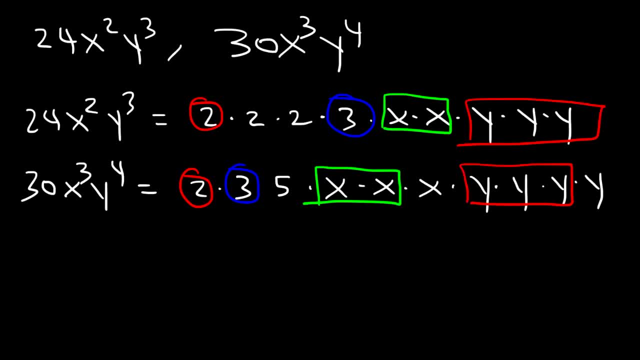 And 3y variables. So the GCF is going to contain a, 2,, a, 3, 2x variables and 3y variables. So 2 times 3 is 6.. 2 times x is x squared. 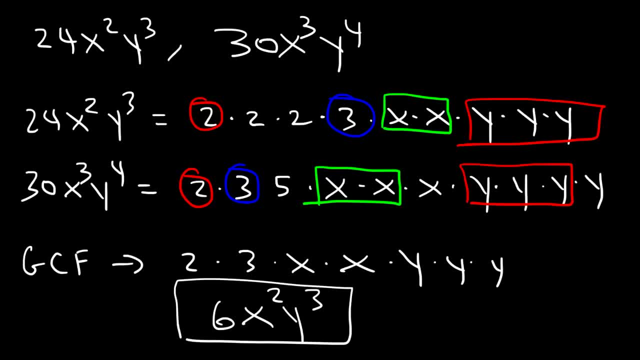 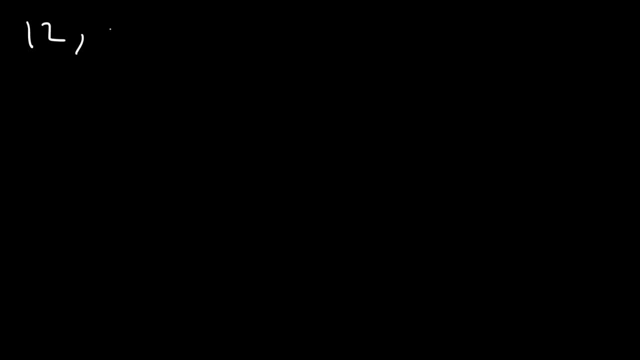 3y's represent y cubed. So this is the greatest common factor between these two monomials. Now what about finding the GCF between three numbers, Let's say 12,, 18, and 20.. Now, the process is the same. 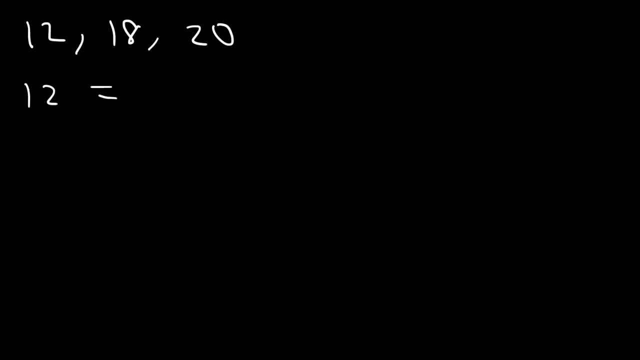 It's simply longer. The prime factorization of 12 is 2 times 2 times 3. And 18, that's 3 times 6. And 6 is 3 times 2.. But let me write it in ascending order. 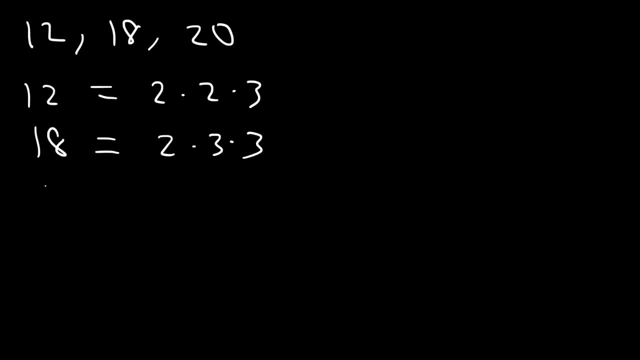 So the prime factorization of 18 is 2 times 3 times 3. And for 20, it's 4 times 5. And 4 is 2 times 2.. Now, once you have the prime factorization of all three numbers, identify what's common to it. 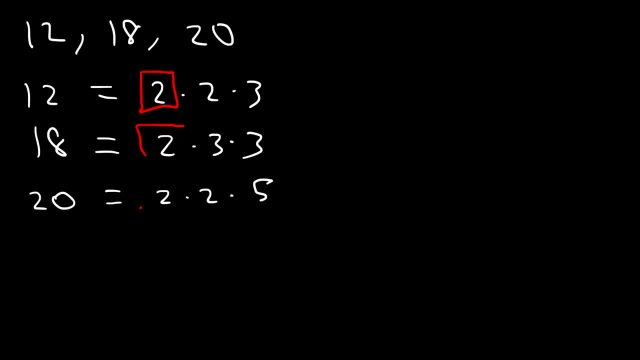 So each number contains at least one 2.. And not every number has a 3 or a 5., But all numbers do contain at least one 2.. So therefore, 2 is the GCF between 12,, 18, and 20.. 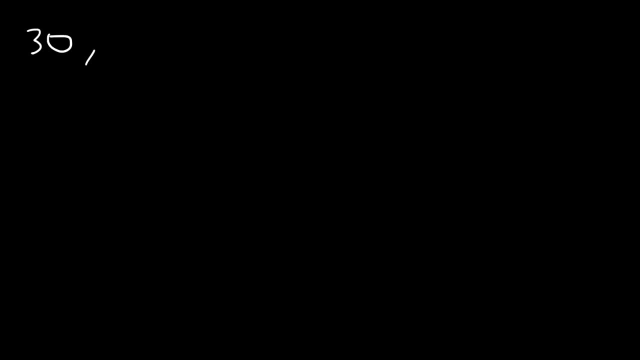 Now what about between 30, 48, and 56? What is the greatest common factor between those three numbers? So 30 is 5 times 6, or 6 times 5.. And 6 is 2 times 3.. 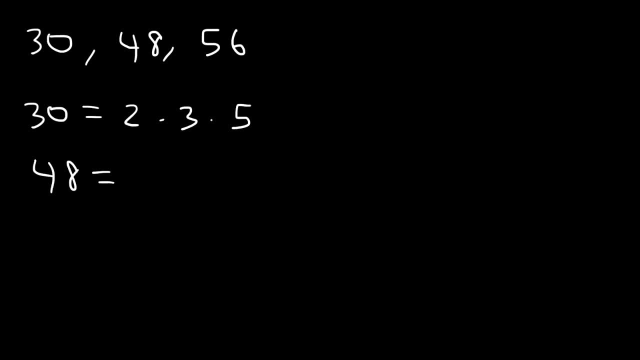 So that's the prime factorization of 30.. The prime factorization of 48 is 2 times 24.. And 24 is 2 times 12.. And 12 is 2 times 6.. And 6 is 2 times 3.. 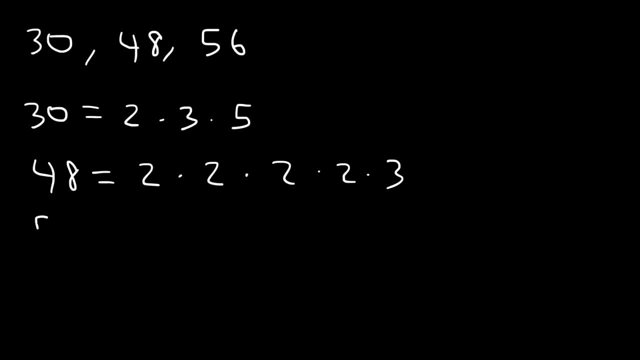 So that's the prime factorization of 48.. And 56 is 2 times 28.. 28 is 2 times 14.. 14 is 2 times 7.. Now let's find out what's common to everything. 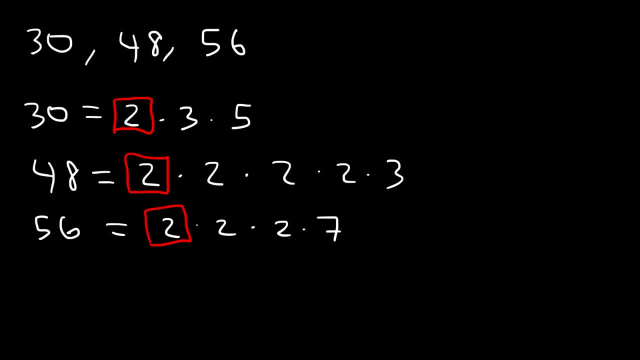 All three numbers contain at least one 2.. Not all of them contain a 3.. 56 doesn't have a 3 involved, And not all of them contain a 5 or a 7.. So, once again, the GCF is simply 2.. 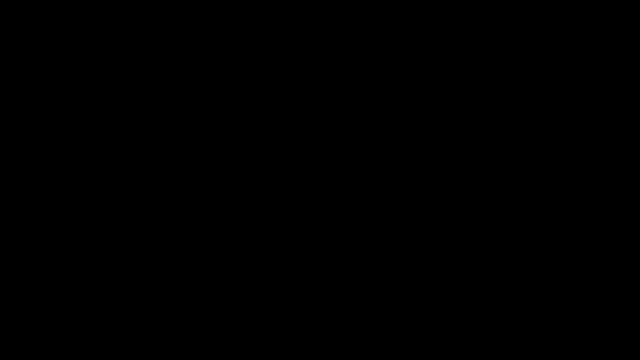 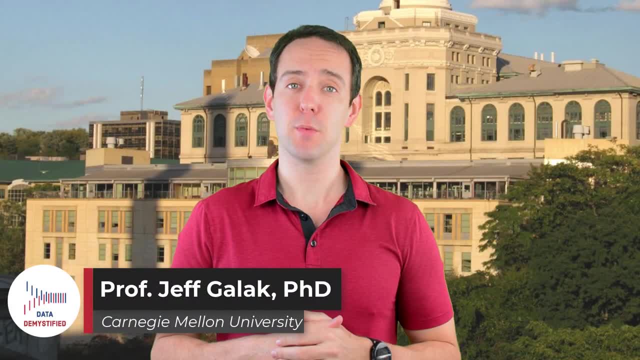 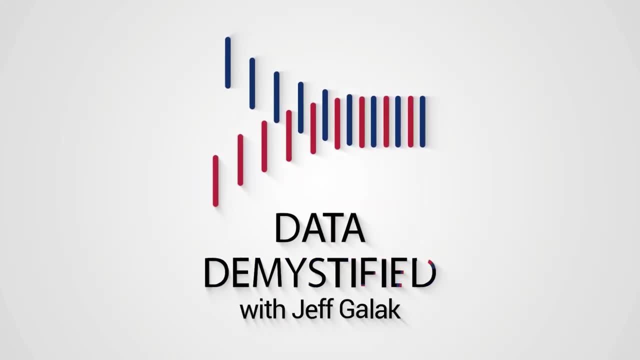 Welcome to Data Demystified. I'm Jeff Gallack and I'm on a mission to equip you with the information you need to thrive in our data-rich world. If you've ever seen a news story about a scientific study, you've probably heard something.